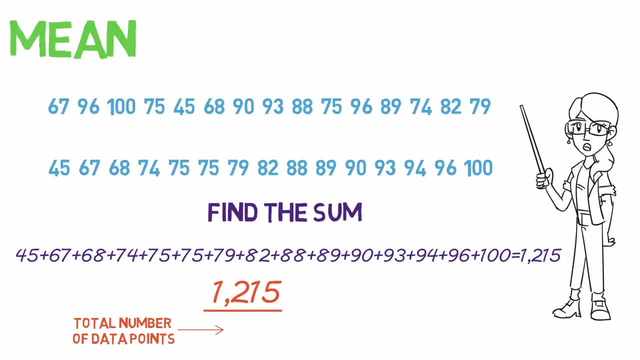 divide it by the total number of data points. We have 15 test scores. so we divide 1,215 by 15, which you can divide by the total number of data points. So we have 15 test scores, so we divide. 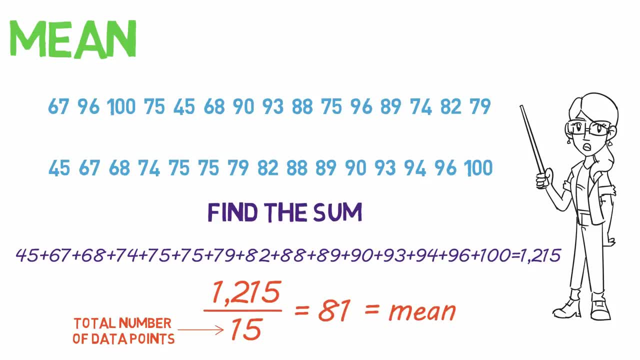 which you can divide by the total number of data points. So we have 15 test scores, so we divide equals 81. And this is our mean. It won't always come out so clean and will likely have several decimals, so you'll have to round it off. 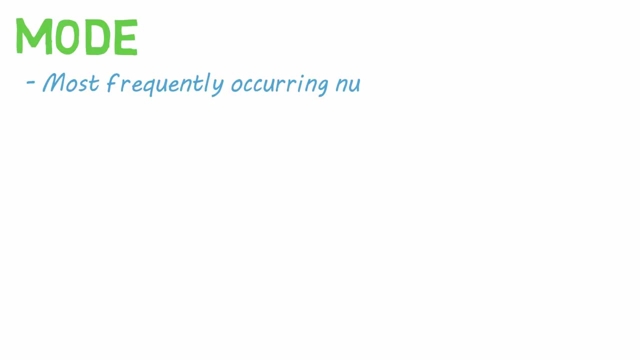 Let's do the mode next. The mode is the most frequently occurring number in a data set. It's easiest to find this when all the numbers are numerically ordered from least to greatest. In this set we only have one number that is repeated more than once: 75. So that is. 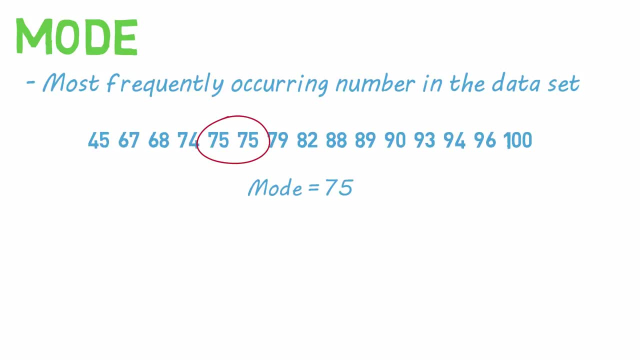 our mode. If a data set has no repeat values, so every number appears only once, then there is no mode. A data set can also have multiple modes. For example, if we have a data set like this, the modes would be 15 and 21, because they are the most repeated numbers, with three. 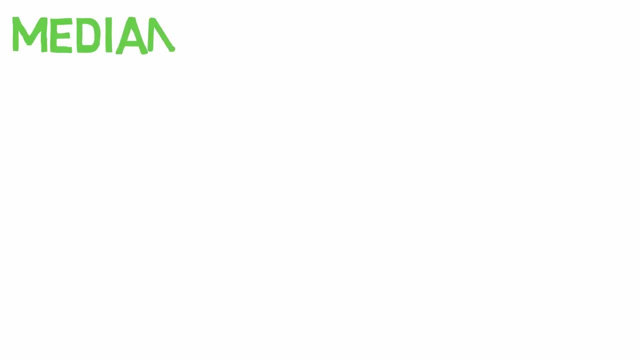 each. Now on to the median. The median is the middle value. Again, you want the numbers ordered numerically from least to greatest. Let's do the mode next. The median is the middle value. Again, you want the numbers ordered numerically from least to greatest. 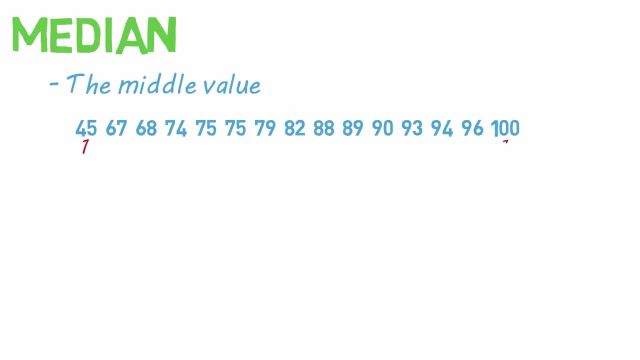 The easiest way to find the median is to count from the outside in like: so If you're left with a single number in the middle, that is your median. However, if you have an even number of values, you'll end up with two numbers in the middle, So you'll 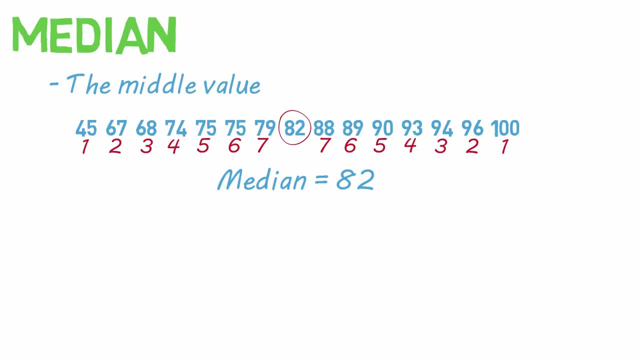 have to take the mean of those two numbers by adding them together and dividing by two. This will give you the median. Here's a quick example. In this example, 7 and 9 are both in the middle. So we add those together to get 16, and divide 16 by 2 to get 8.. And this is our median for this data. 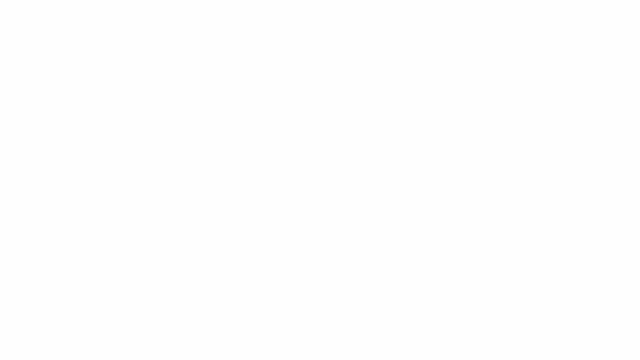 set. I want to give an honorable mention here to the range. It's not really an average, but you may be asked to find it. It's simply the difference between the highest and lowest values. So take the highest value and subtract the lowest value from it, And that's the range. 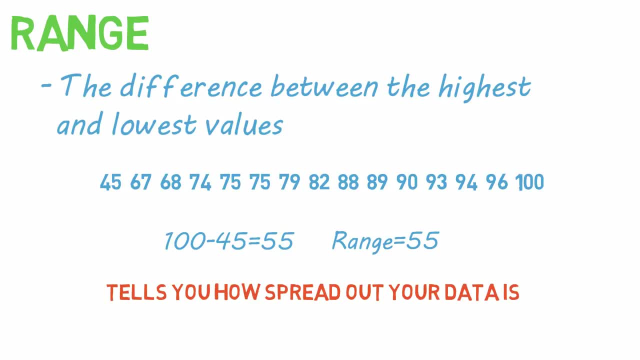